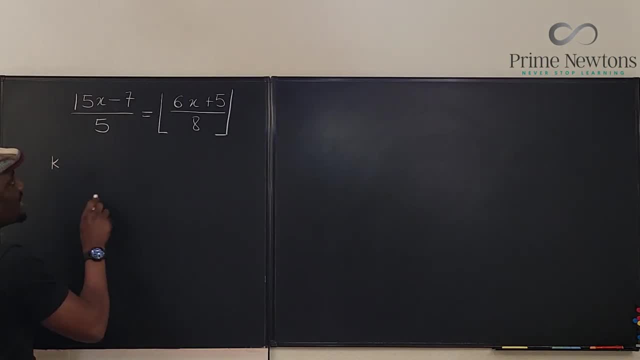 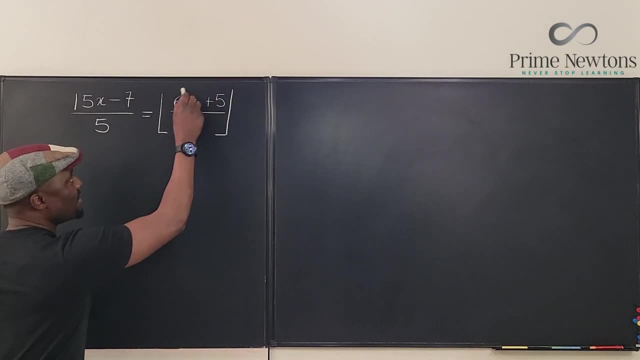 is equal to k. We know that this floor is equal to K, But when you compare it to what is inside, it is less than or equal to six X plus five over eight, And this is always less than its own ceiling, which can be written, in terms of the floor, as K plus one. 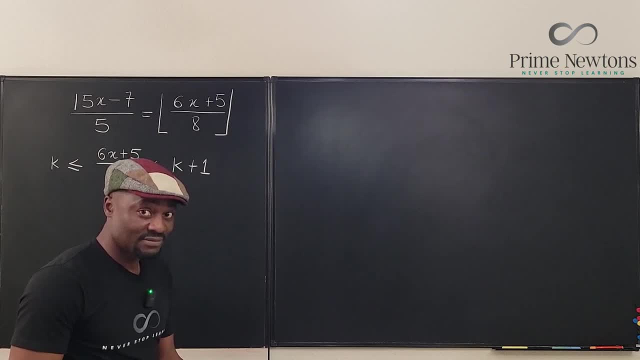 So this is the first thing that we need. We also know that 15 X minus seven over five is K, because that is the floor of this side. So those are the two things you need and you'll be able to get your answer. So let's clean this up. 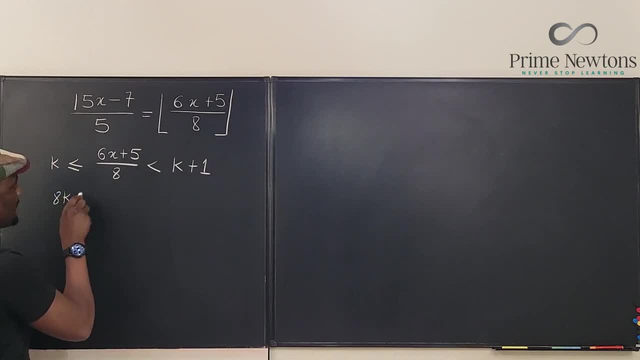 Let's multiply everything by eight, So we have eight K is less than or equal to six X plus five, and it's less than eight K plus eight. We can remove this, five subtract five, We have eight K minus five is less than or equal to six X. 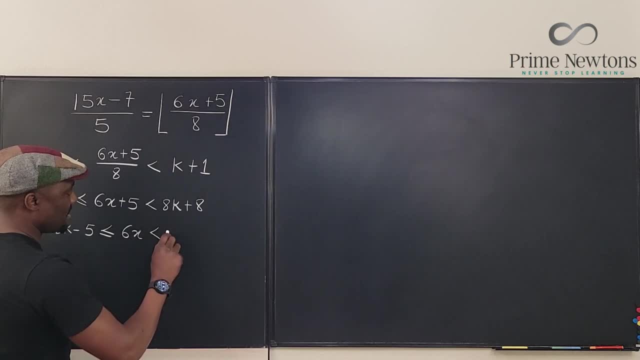 and that's less than. if we subtract five from here, you're gonna have eight K plus three. And then you divide by six. you have eight K minus five. divided by six is less than or equal to X, and that's less 8k plus 3 divided by 6.. So this is an essential part. Let's mark it. We also 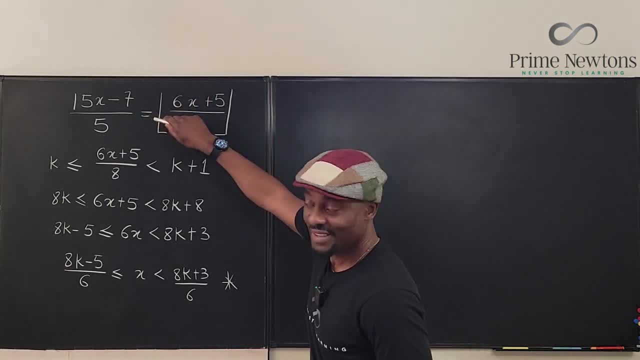 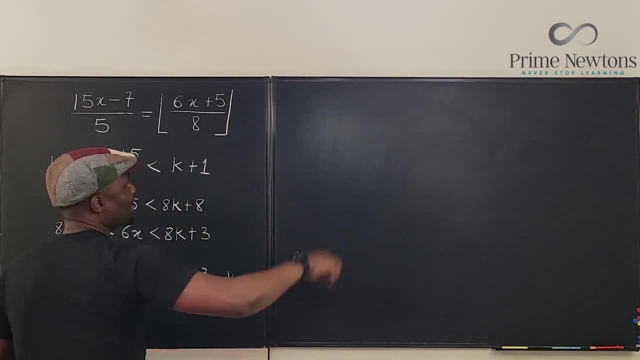 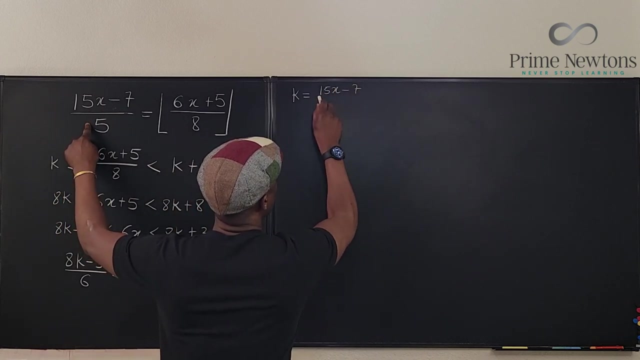 know that k is equal to this, So we can as well say that. let's write it here. k is equal to 15x minus 7 over 5.. So if we multiply we have: 5k is equal to. so what? 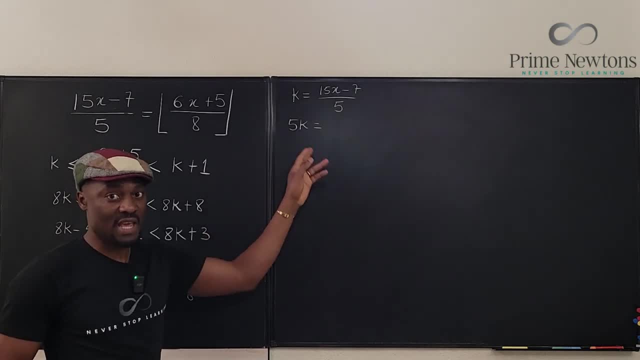 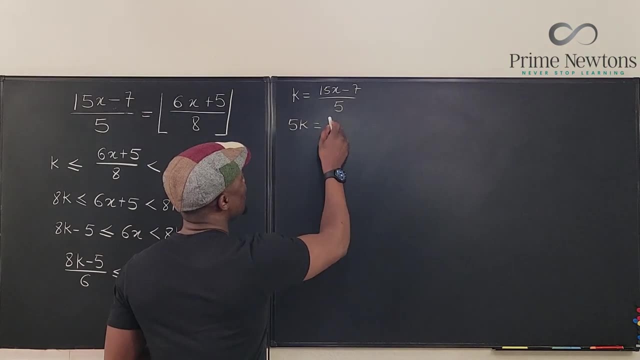 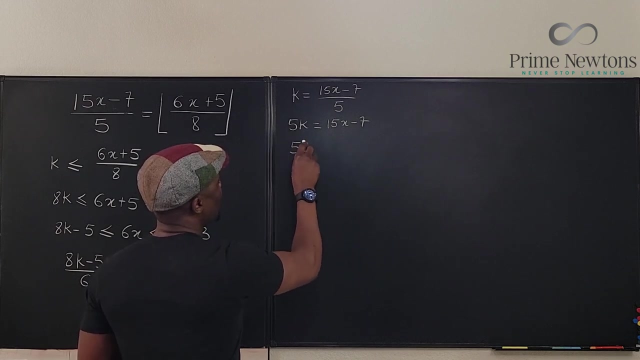 we're trying to do here is we need to write x in terms of k. Here we have an inequality, but we need an equation. So it's going to be: 5k is going to be 15x minus 7, which shows that 5k- let's say 5k plus 7- divided by 15, will be equal to. 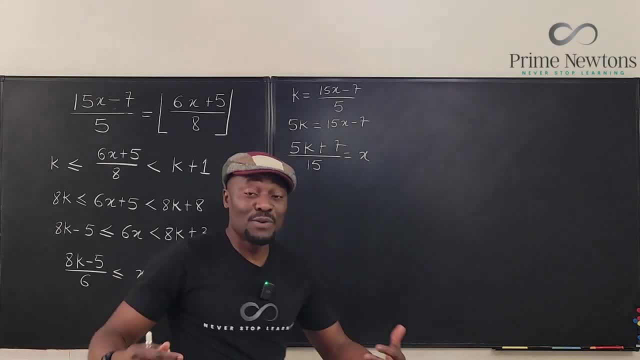 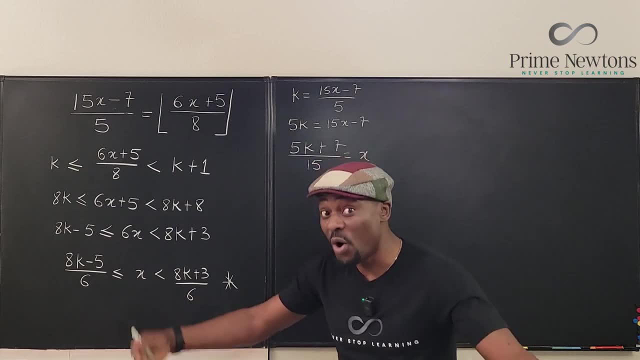 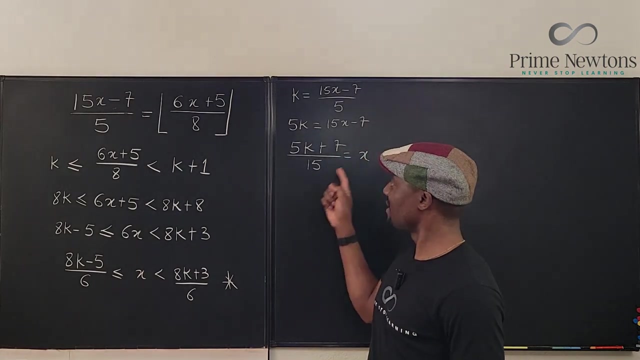 x. Now, once you've gotten to the point where you've written x in terms of k and you have an inequality, or you have an inequality or inequalities connecting x with k, you're ready to start solving, Because now I know this is my x, but I 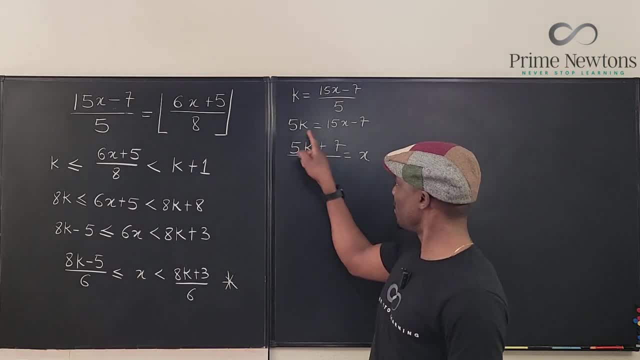 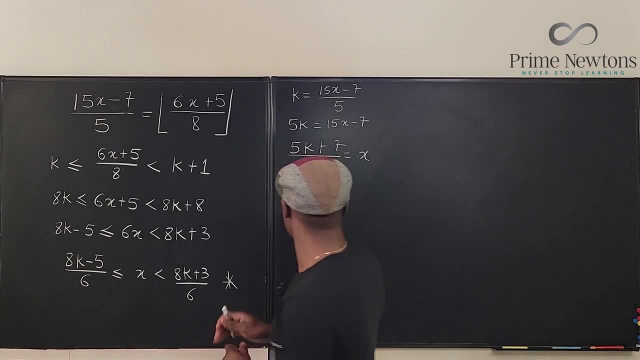 can do x, I can do x and k, I can do k and k. So I'm going to take this and put it here in the middle, so that my inequality in essence is going to be: let's write it therefore, let. 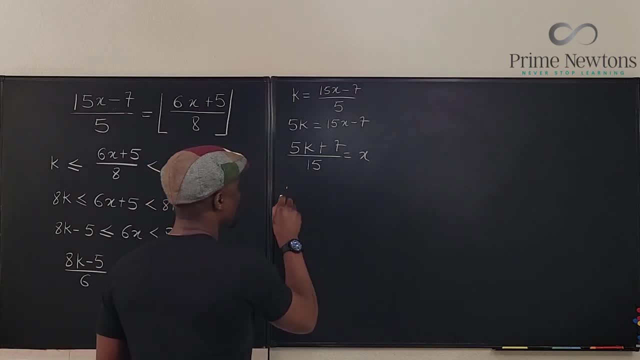 me go back here. No, that's going back. I don't want to go back. So we can say: therefore, 8k minus 5 over 6 is less than or equal to x. but this is my x, It's going to. 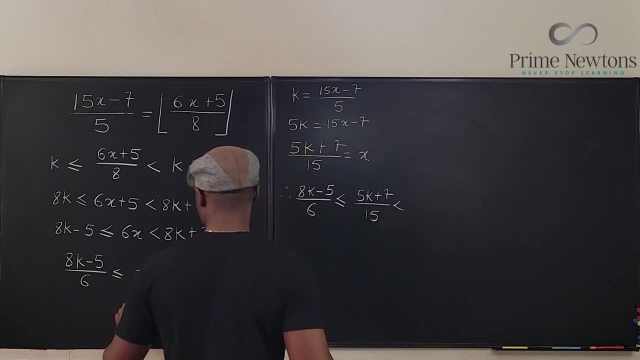 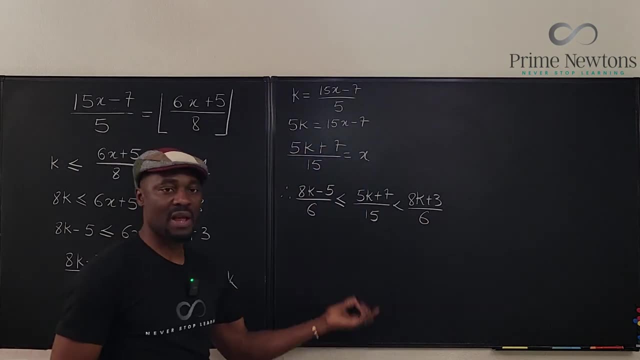 be 7 over 15, and that's less than 8k plus 3 over 6.. So now you can solve two pairs of inequalities. But before we move on, I'd like to clear these fractions, So I'm going to. 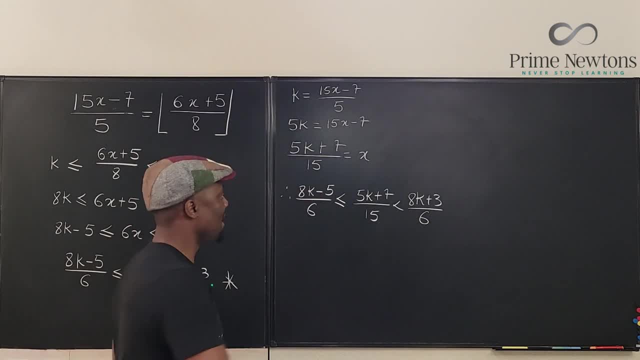 multiply every part here by 30. Okay, multiply this by 30, by 30, by 30, you're going to end up with 5 here. So this is going to be 40k minus 25.. It's less than 8k plus 3 over. 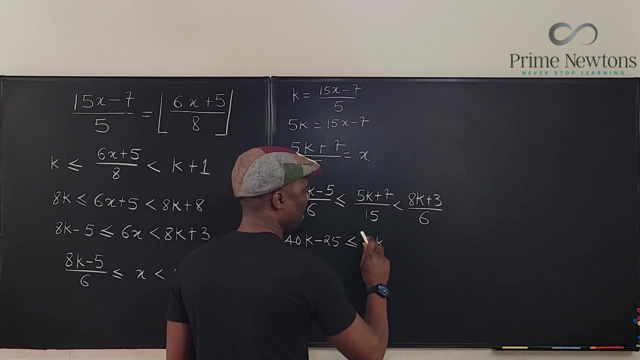 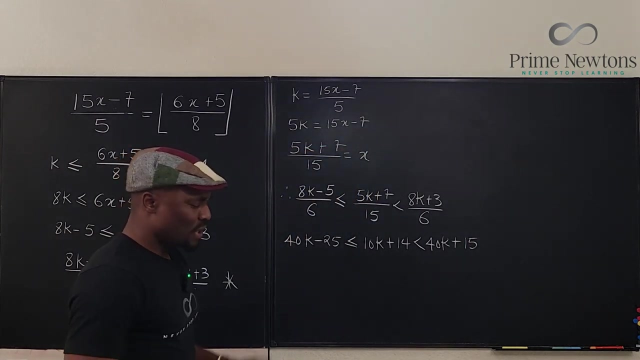 7, or equal to multiply by 30,, you have 10k plus 14, and it's less than 5.. That's 40k plus 15.. Okay, What are we looking for? again, We're looking. we want to know what k is. So. 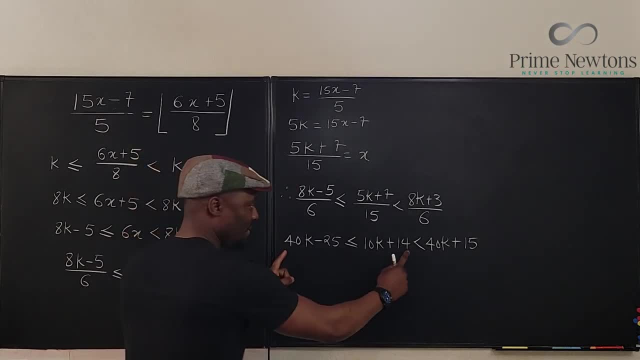 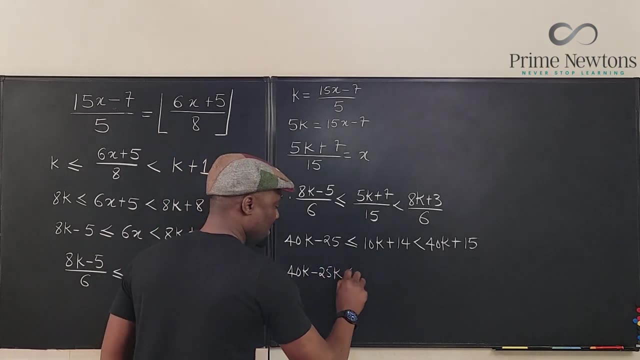 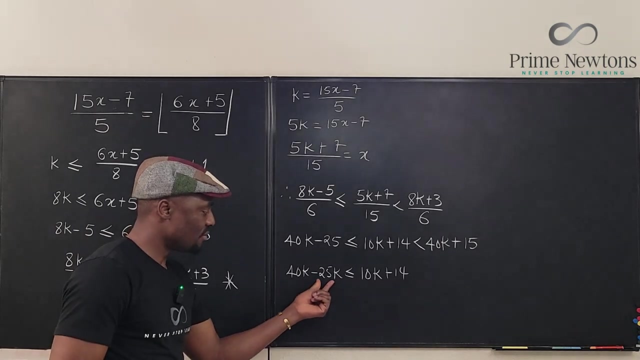 let's now have two separate inequalities. We're going to focus on this one. So we have 40k minus 25.. 40k minus 25k is less than, or equal to, 10k plus 14.. If I bring this 10k here and move, 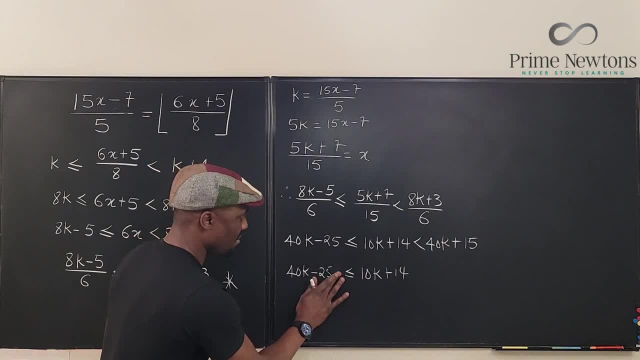 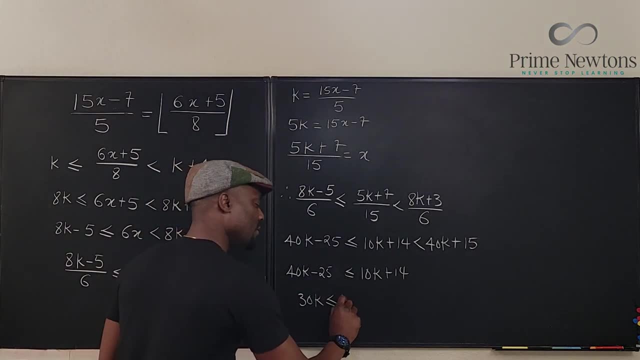 this over to this. sorry, this is just 25, and I move this 25 over to the other side I'm going to end up with: 30k is less than, or equal to 39. So that k is less than or. 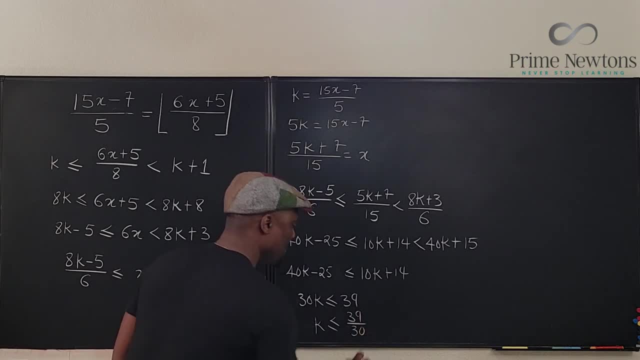 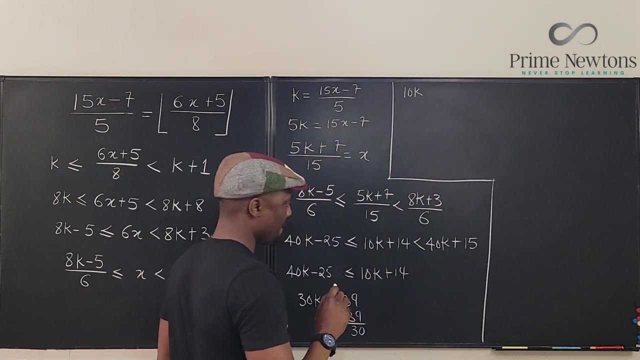 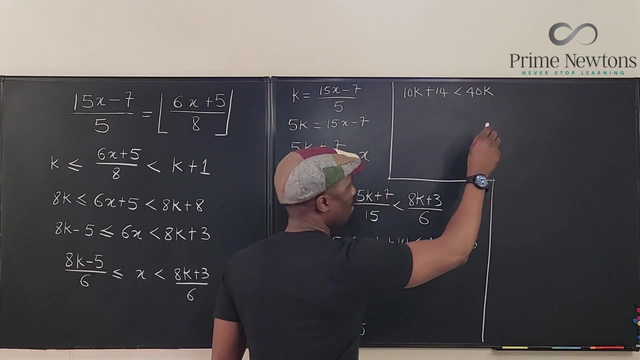 equal to 39 over 30. So this number is actually greater than one, but it's less than two, Ta-da-da. Okay, let's solve the second part of the inequality. We're going to say that 10k plus 14 is less than 40k plus 15.. So that: 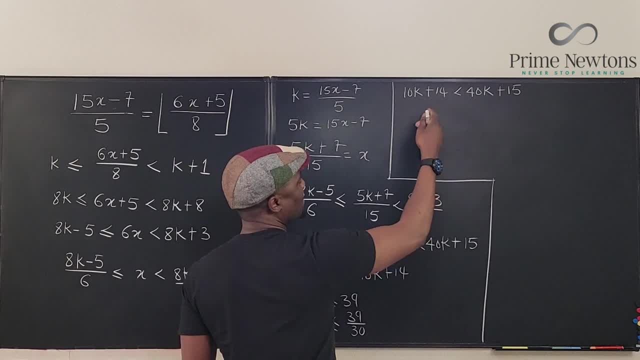 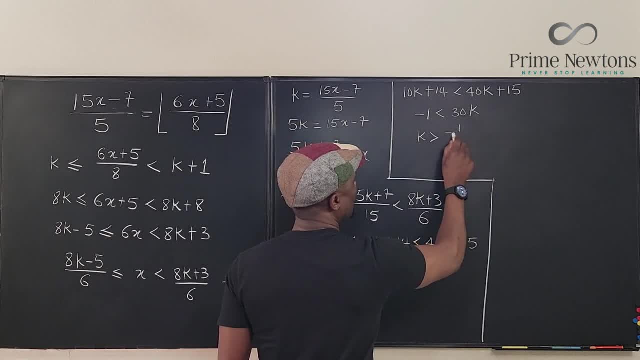 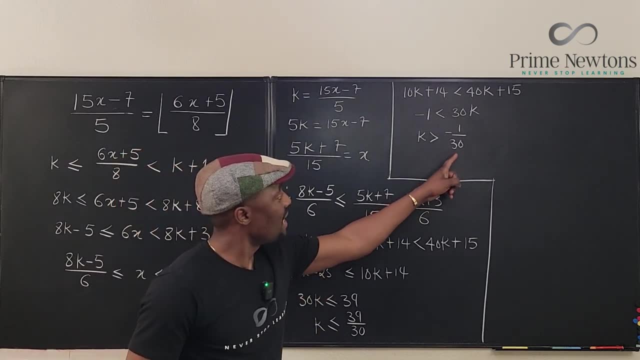 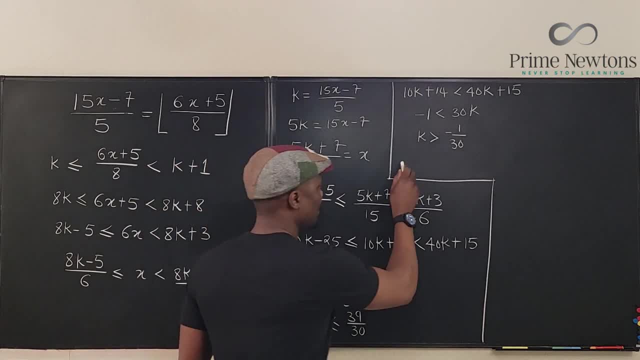 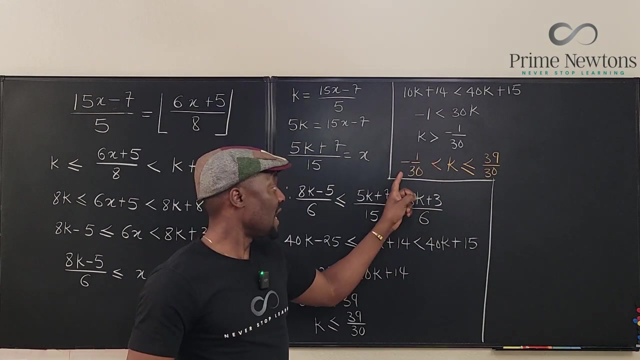 and we have a number that is greater than k. so we can say: finally, let's write it with this one. so we know that negative 1 over 30 is less than k and k is less than or equal to 39 over 30.. Based on this result, the two integers that are in this range are 0 and 1.. Those are: